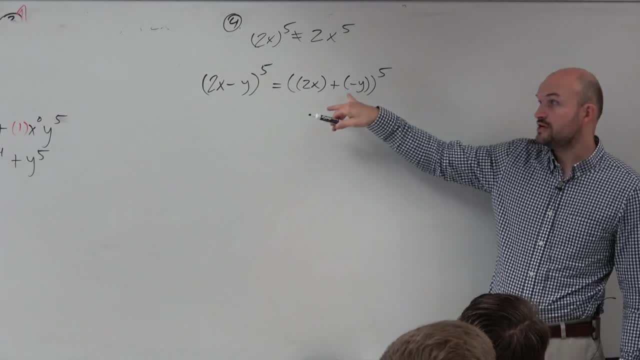 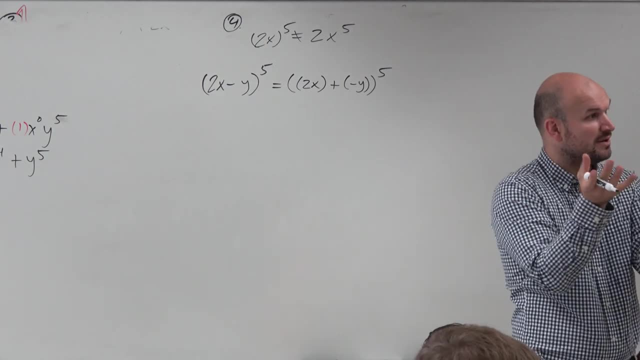 around each term. I'm going to change this to a plus and negative y, so I know that there's a negative 1 as my coefficient, Because- notice- the formula for the binomial expansion was the sum of two values, So I'm going to rewrite it as a sum. Now let's go and use the binomial. 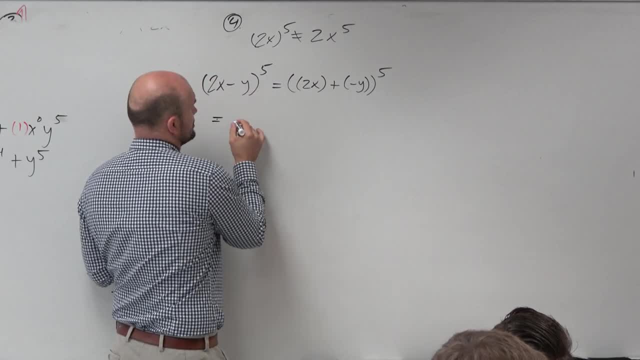 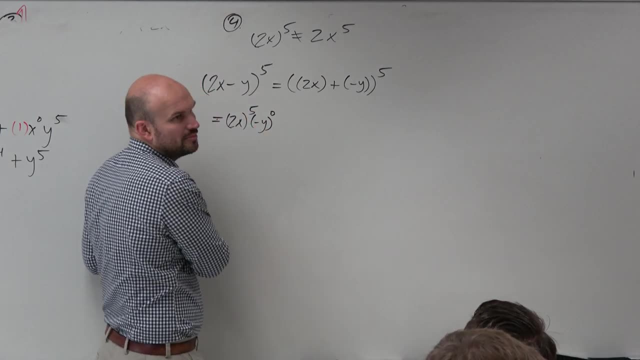 theorem to identify the powers. So I'm going to have 2x parentheses to the fifth power. You don't really need to write this first term to the zero power, I'm just writing it so you guys can see the pattern. But in reality, guys, 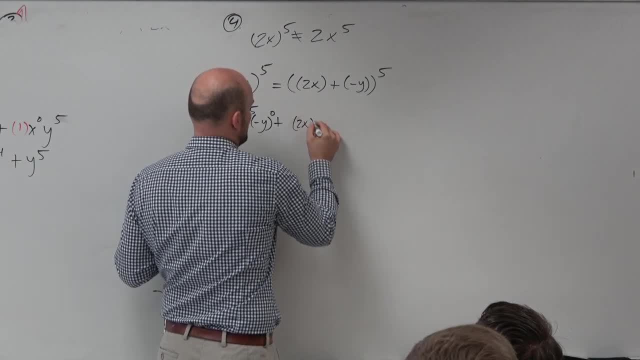 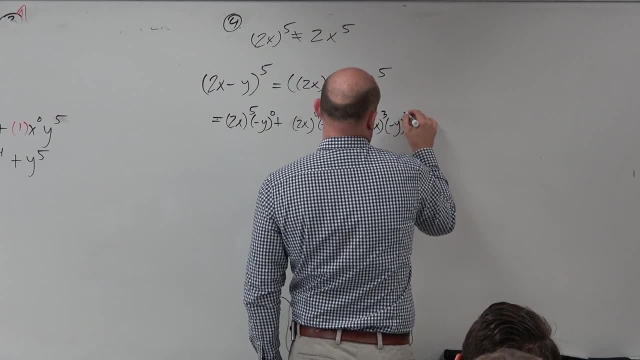 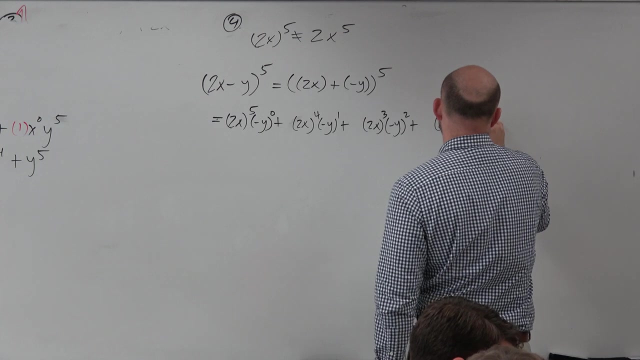 if you don't want to write that number, by all means you can skip that portion And you can see there's a lot of. let's see that's going 2, negative 1, 2 to the fifth, negative 1 to the third. 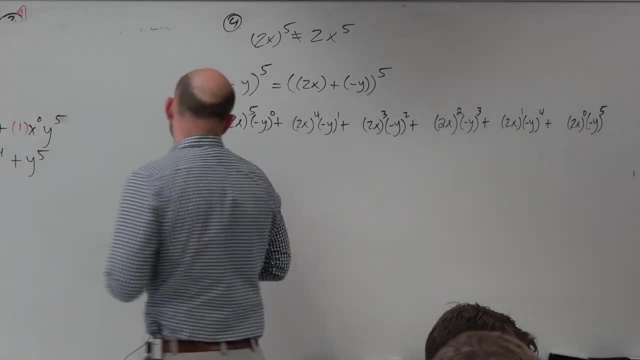 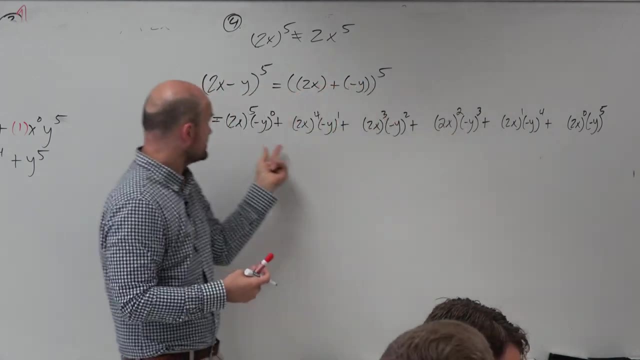 Woo, OK, But again, do you see the first term, that 2x going into ascending powers- Right? Do you see the second term, starting at zero and going into ascending powers- Right? It works for all of them. 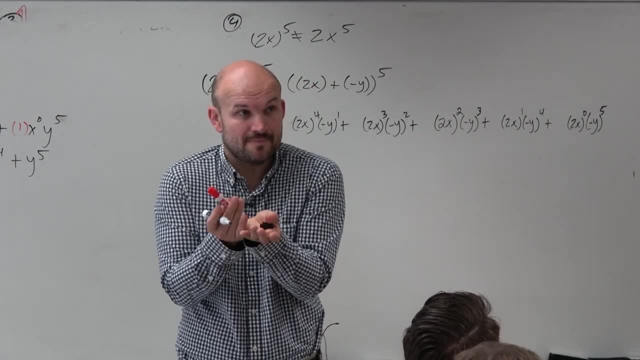 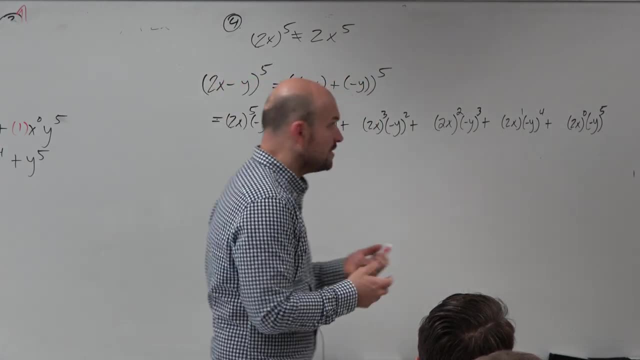 Just keep on going up, Just start with the same thing every single time. Yes, time. Now. the real question is: well, what about the exponents? Where's that fifth row in here? Well, the fifth row again is just like what. 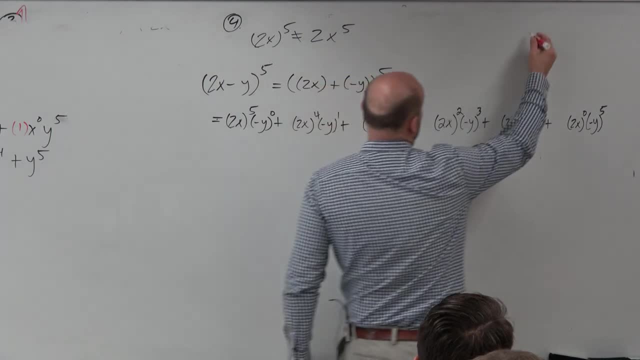 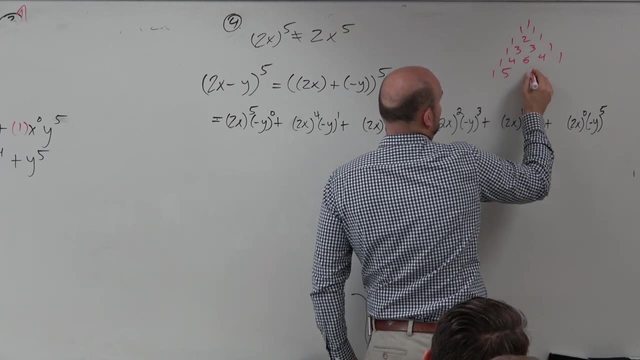 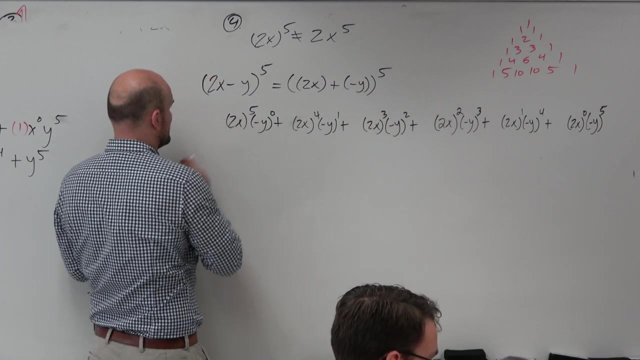 we did in the last one, right? So go through the Pascal's triangle, create it. Here's the fifth row, because that's the second term, Right? Oh, good thing. So therefore, make sure you recognize that those are the coefficients here. 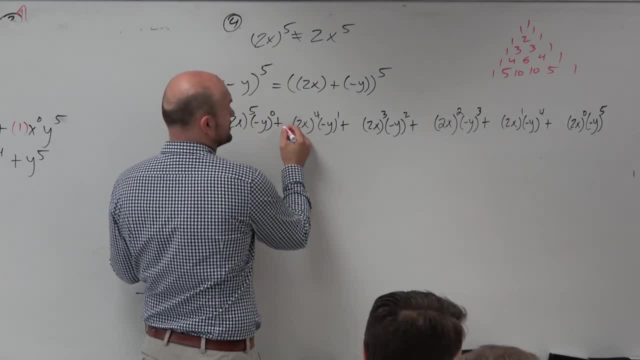 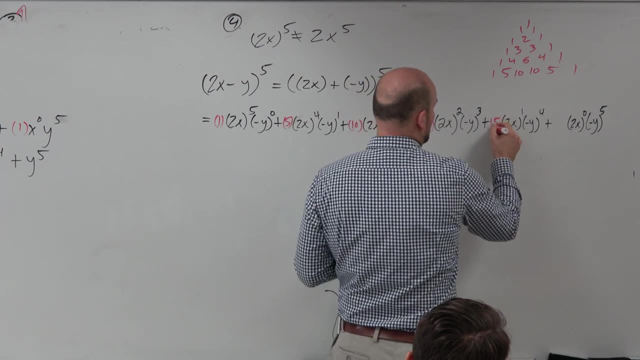 But the problem or the thing that I want to make sure you guys understand here is that doesn't mean that's what the coefficients are, Because the terms also have coefficients Right. So when you show your work, like when we do our work, 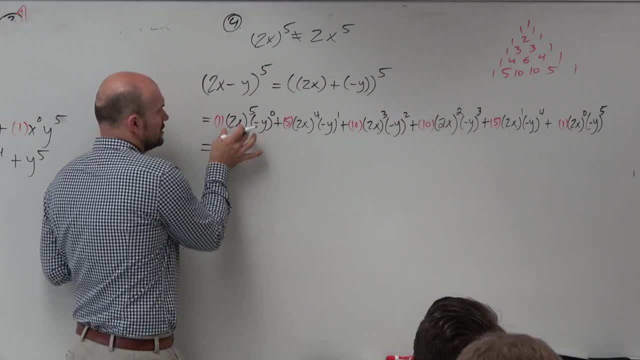 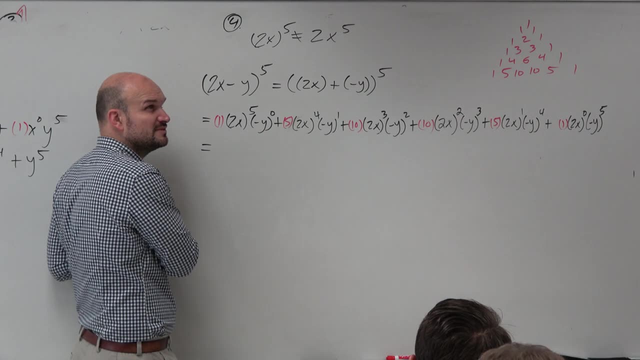 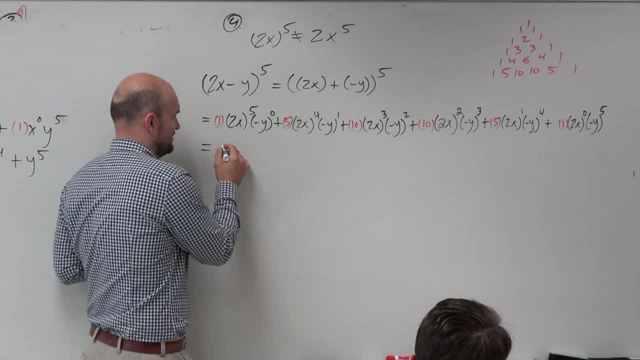 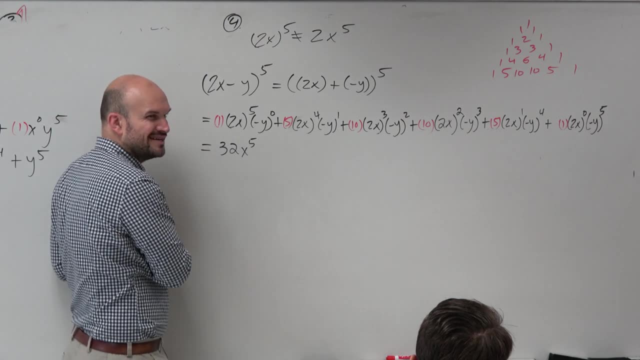 That's going to give me 32x. to the fifth Negative. anything raised to the 0 power is 1, so I'm just going to leave it off right. The next one, This one, starts to get important. I'm just going to do two steps. 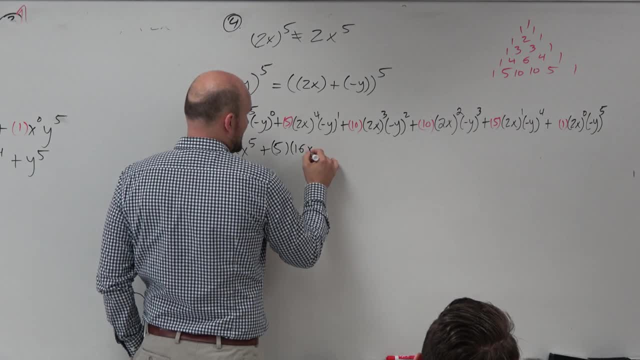 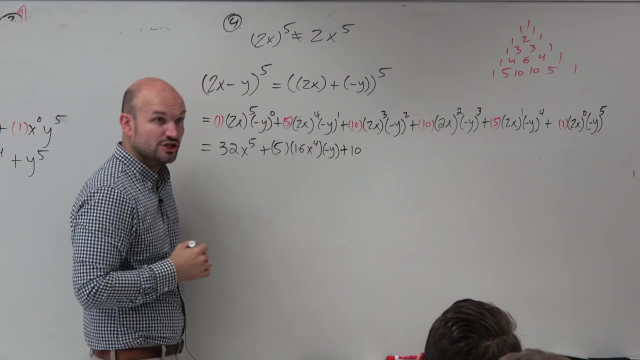 I'll do 5.. 2x to the fourth is going to be a 16x to the fourth. Negative y to the first is a negative y Plus 10.. 2x cubed is going to be 8x cubed. 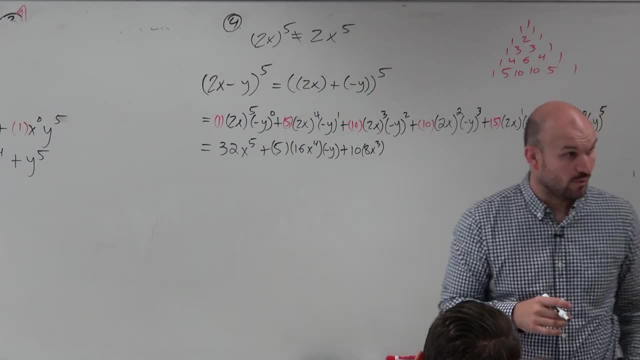 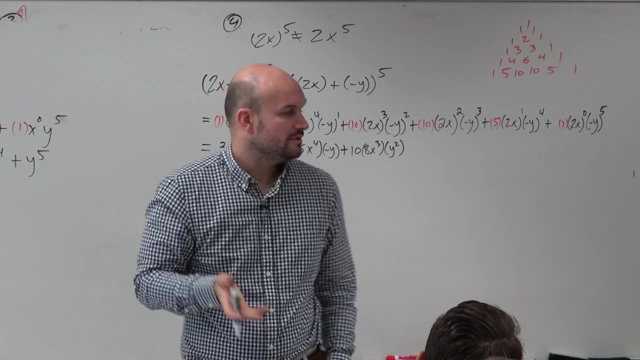 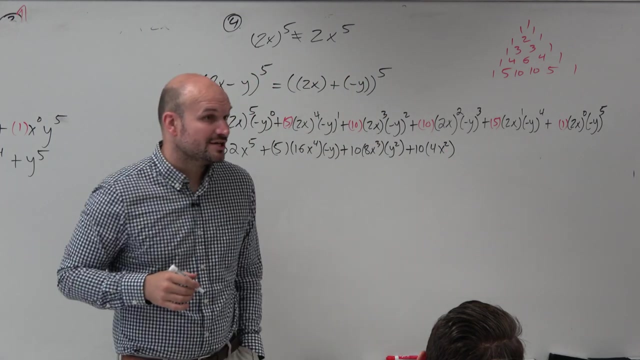 Negative y squared Is what Positive y squared Right. Remember, whenever you have a negative term raised to an even power, it's positive. We did that last chapter. 2x squared is 4x squared. Negative y cubed is: 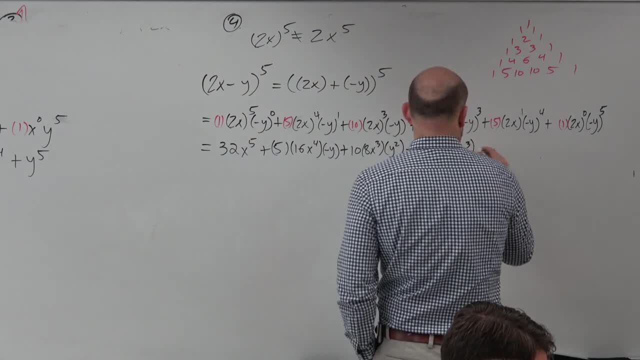 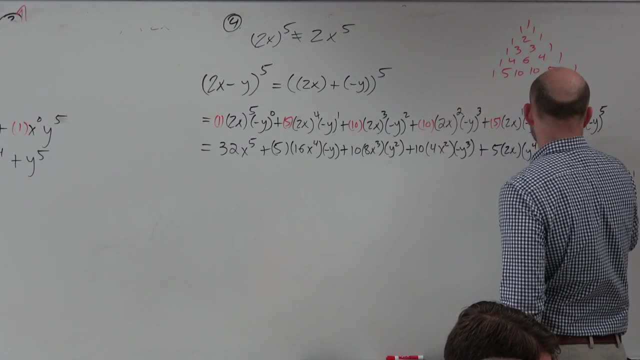 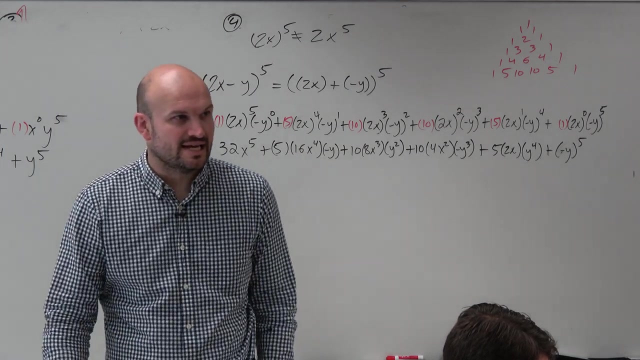 Negative, Negative y cubed plus 5 times, 2x times a positive y to the fourth Plus a Negative y to the fifth. Now you don't need to show all this work, but I'm doing this so you guys can see the second step. 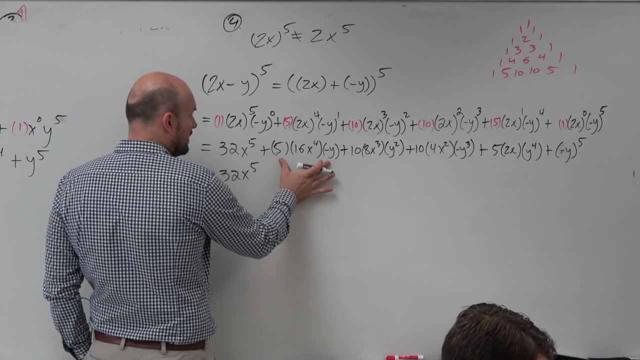 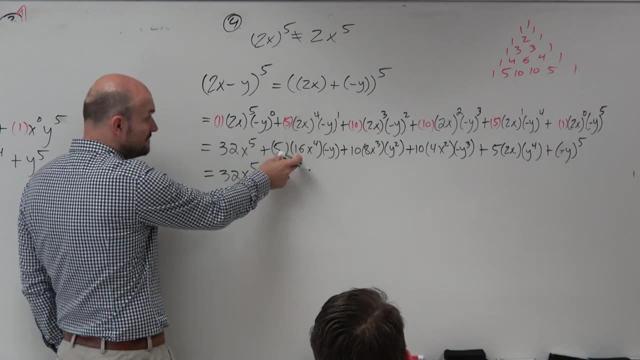 A lot of these you guys could probably do in your head without making a mistake. However, I want you guys to understand that this term, now, 5 times 16, is a negative 80.. Or sorry, 5 times 16 is 80.. 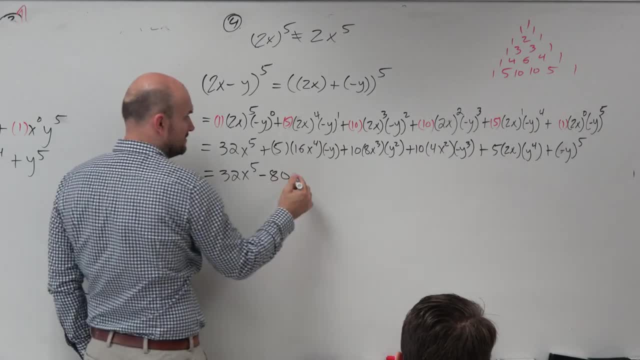 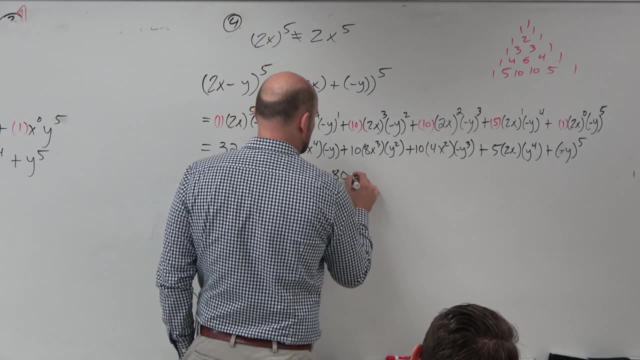 Positive 80.. But then you're multiplying by a negative. That's why you get a negative 80.. 10 times 8 is just going to be positive 80.. Positive 80.. 10 times 4 times a negative, 1 is a negative 40..